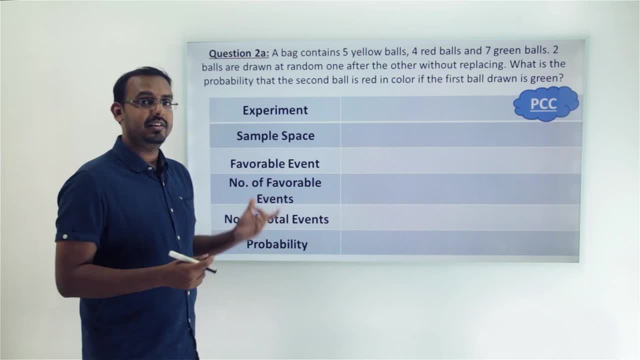 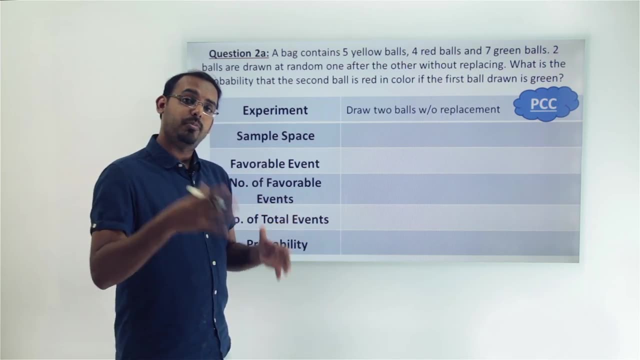 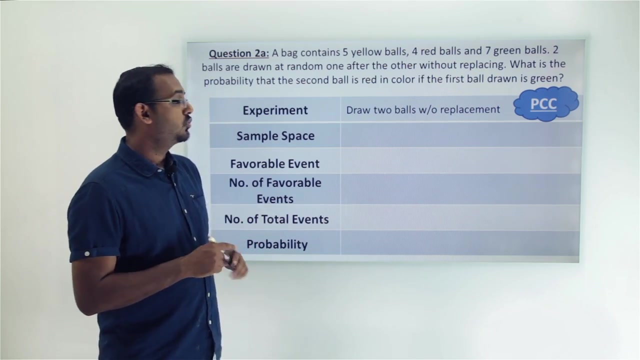 problem, and the first thing that we'll look at is: what is the experiment that we are performing? So the experiment that we are doing here is we take the bag in which we put all these 16 balls, and then we draw out one ball and we keep it aside and then we draw the second ball. So the 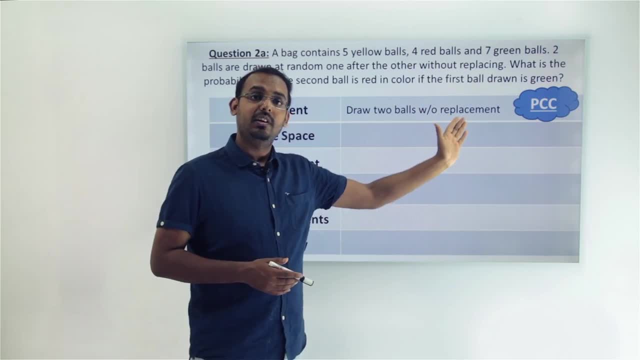 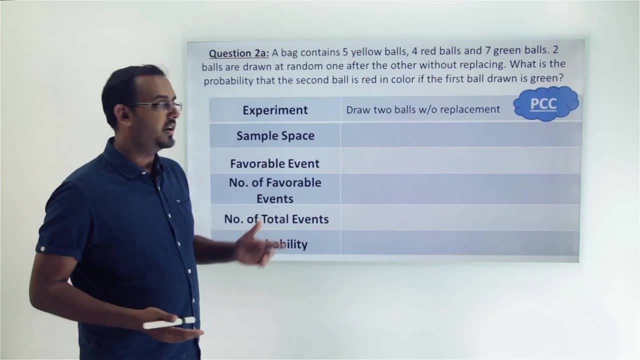 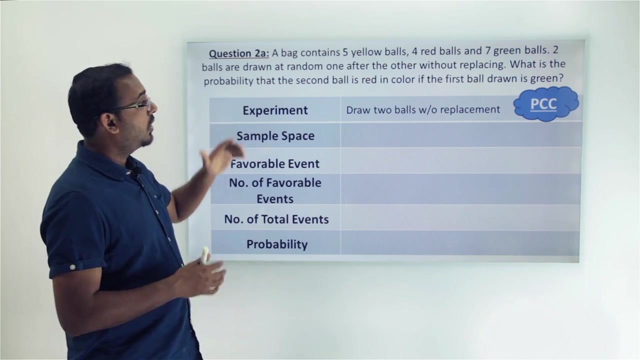 experiment that we are performing is that we draw two balls, without replacement, from the bag. Now the next thing that we figure out is we need to find what is the sample space associated with the experiment. So now here we are, doing two steps. so in the first step, we took out a green ball and 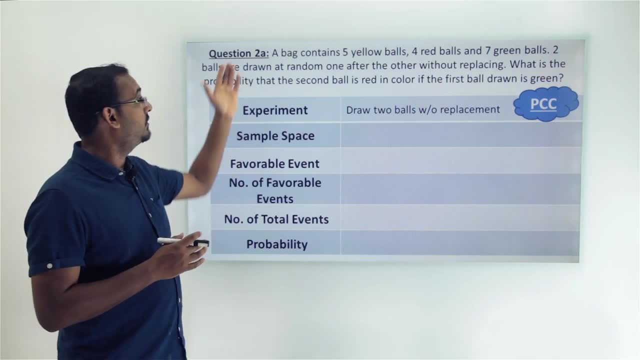 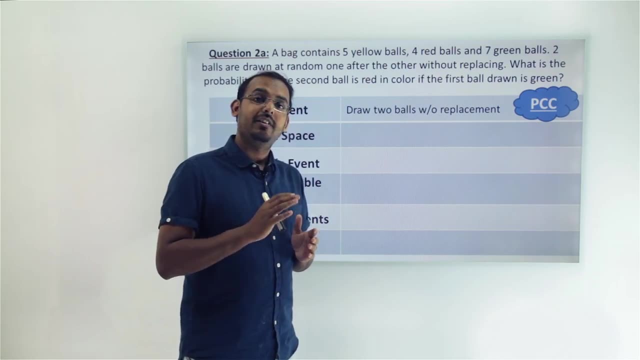 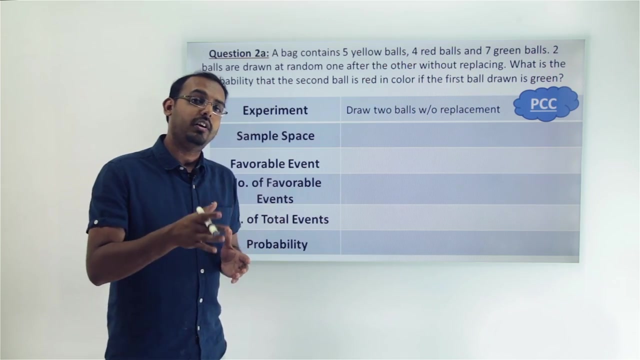 we have kept it aside. So now in the bag we are left with five yellow balls and four red balls and six green balls, because one of the green balls we have taken out and kept aside. So So now think how many balls are there in the bag and what? what forms our sample space? So the 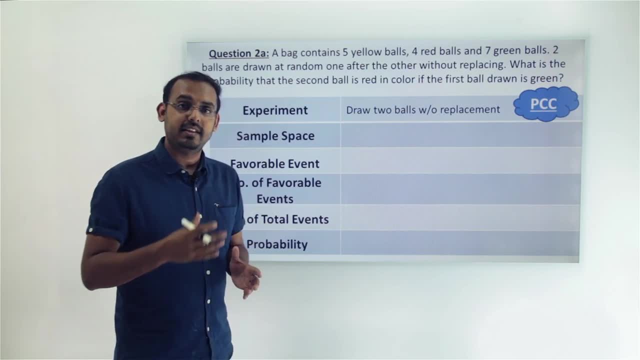 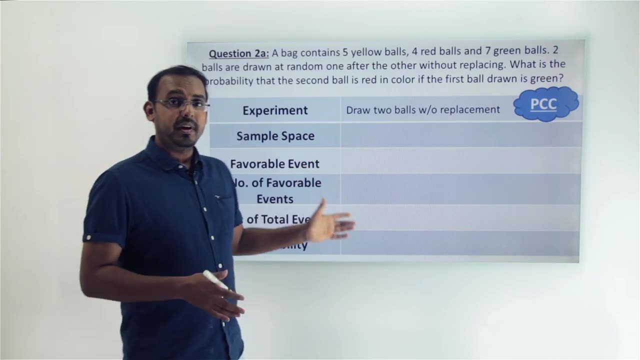 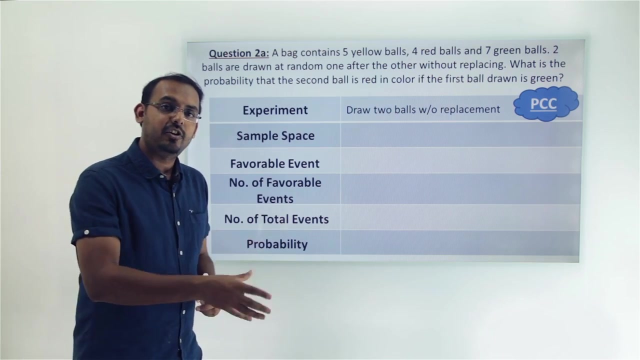 experiment that are performing that we are performing drawing a single ball out of this new bag. so what is the sample space here? so yeah, the sample space is going to be any of the balls, any of the 15 balls which are now present in the bag. so if I draw, 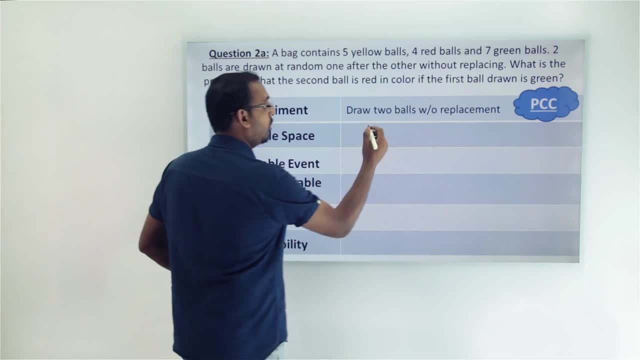 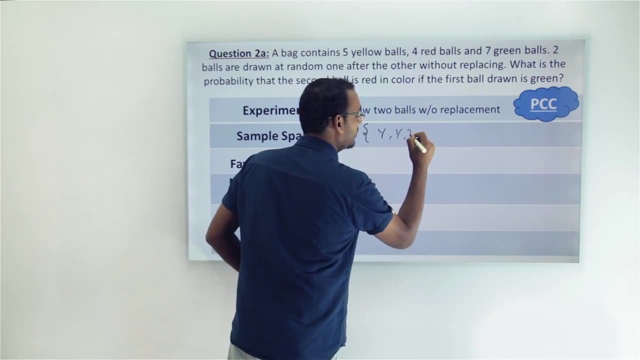 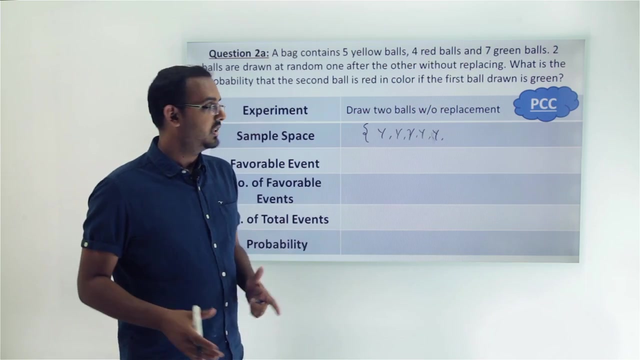 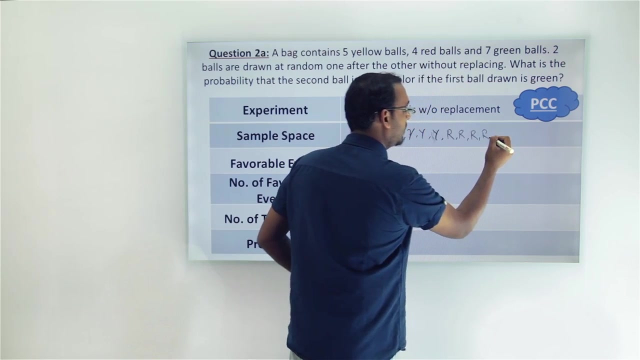 any ball out, i'll be faced with an option of five yellow balls. so there will be yellow ball one, two, three, four and five. so there are five yellow balls now in the bag, and then we have four red balls. so four red balls. and now, since we 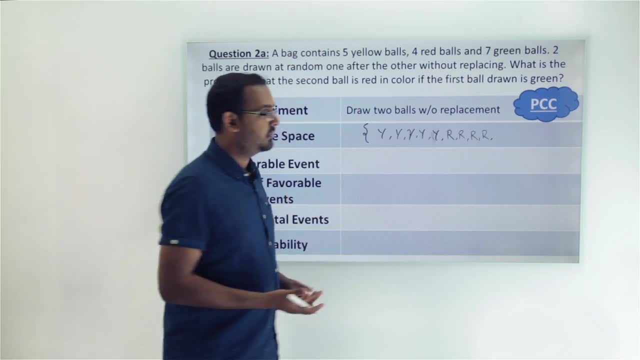 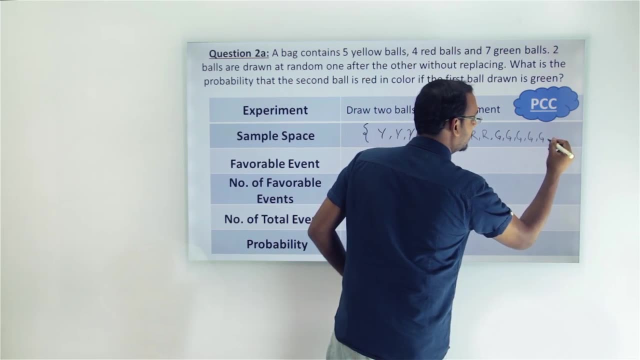 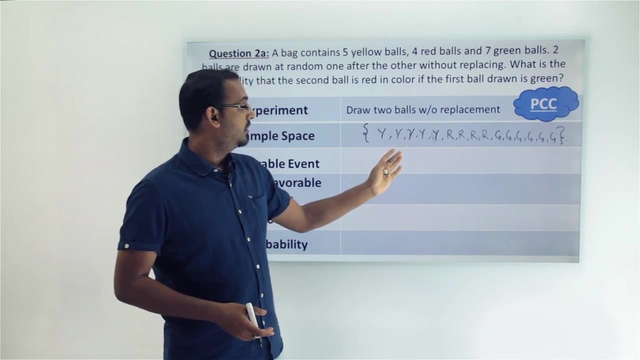 have taken one green ball out already. we have six green balls in the sample space in the bag. so now the sample space consists of these 15 balls, out of which five are yellow, four are red and six are green. so now, what is the favorable event here? so 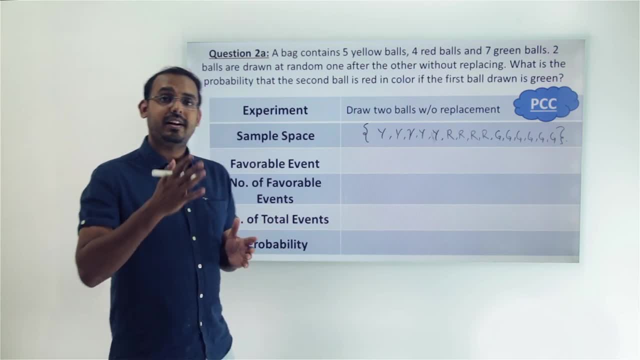 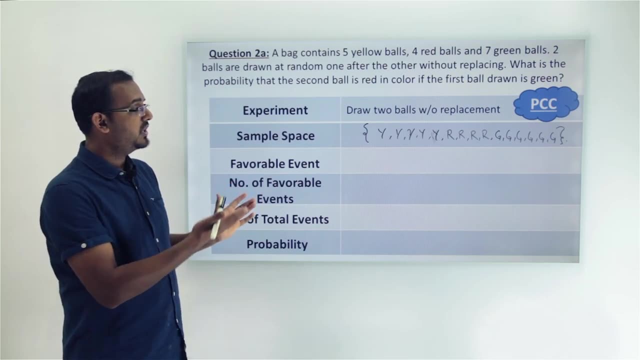 the favorable event now is drawing off a red ball out of the new bag that we have. so so think about it. how many cases are there in which we are drawing a red ball out of the bag, or what is the favorable event? what is the set of favorable? 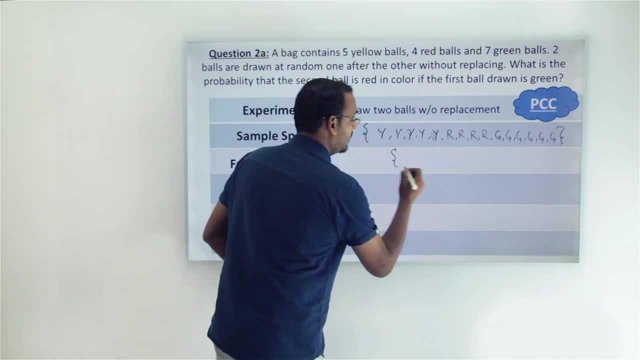 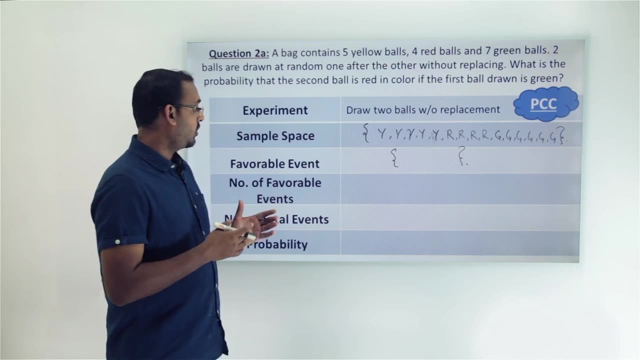 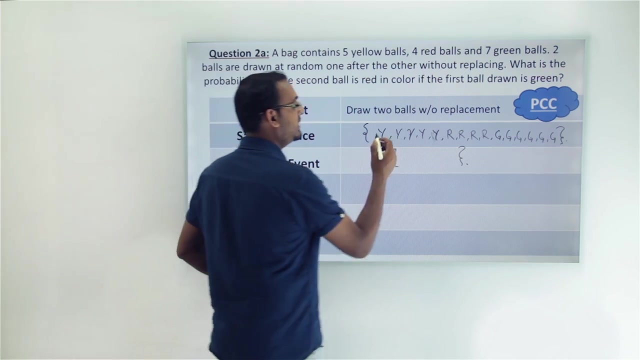 events that we have. so, if you think about it, the favorable event will be drawing any one of the red balls which are now remaining in the bag right. so if we look at the sample space, we can see that these balls are yellow in color. so these form a non-favorable. 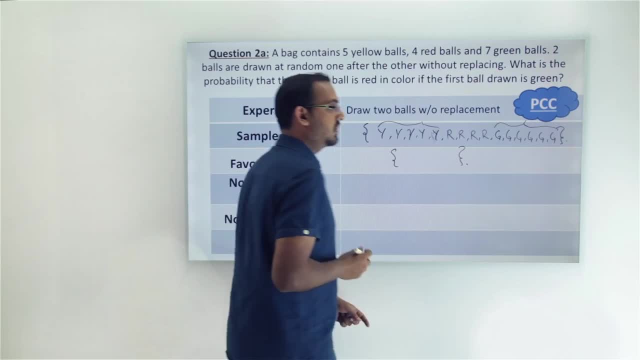 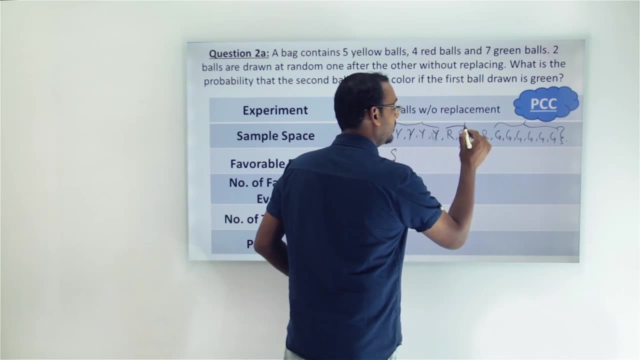 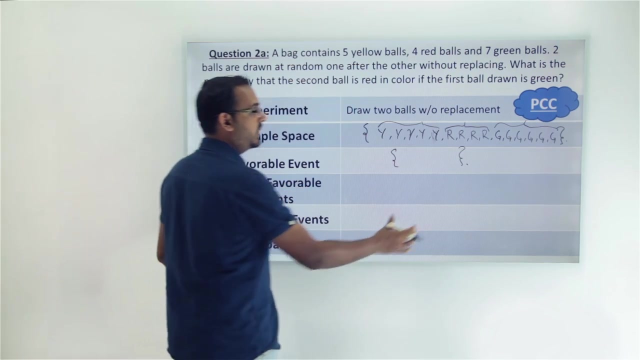 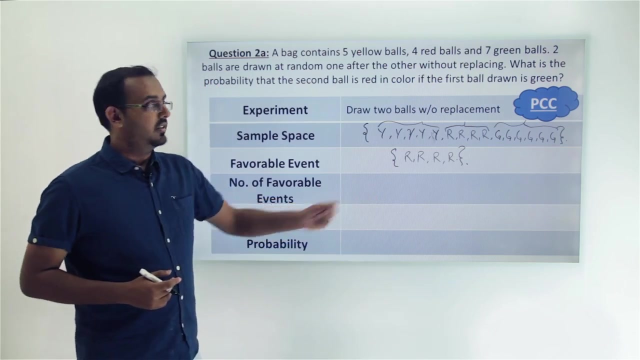 set. so these balls are green in color. so these are also non-favorable to our event. so the favorable balls that we can draw for our event to be true are any of these four balls. so the favorable event set will consist of these four balls which are red in color. so now we have to. 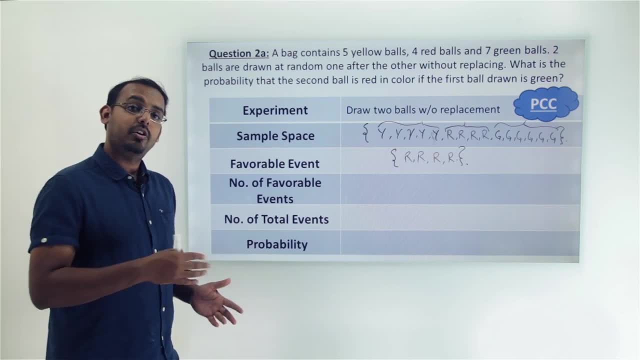 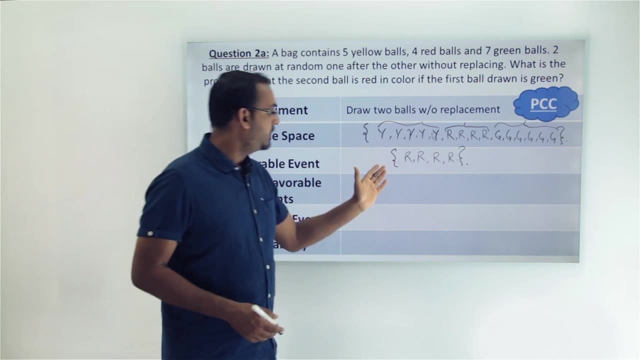 calculate the number of favorable events. so we know that the number of favorable events is the total number of elementary events present in the favorable event set. so if we look at the favorable event set, which we have already figured out, we see that there are four different cases. 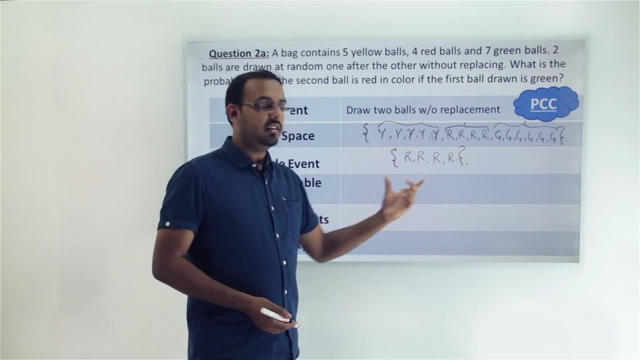 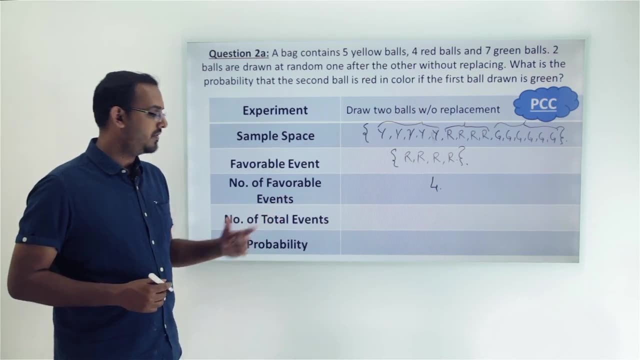 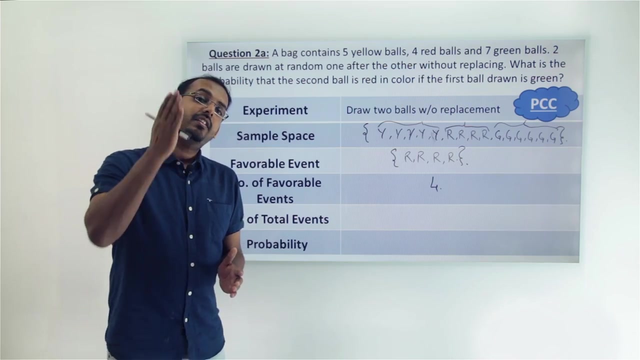 four different elementary events which are present in the favorable event set. so we have four different. so the number of favorable events that we have are four. now think about what, what is going to be the total number of events. so in the first case, when we are drawing out, 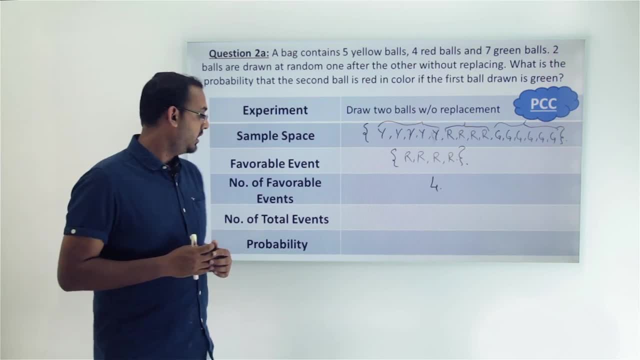 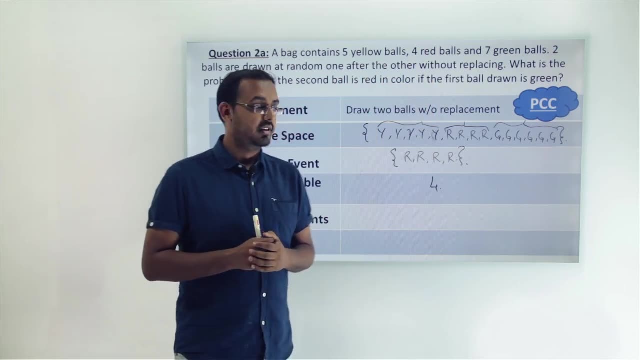 the ball. what was the when we are drawing out the first ball? what was the total number of events? so it was sixteen, right, because initially we had taken sixteen balls, but now, since we have taken out one ball and kept it aside, what is the total number of events? 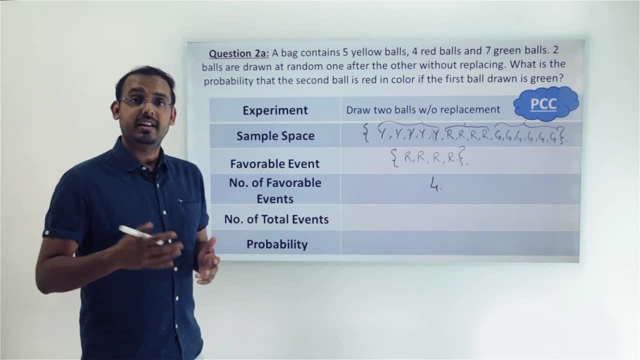 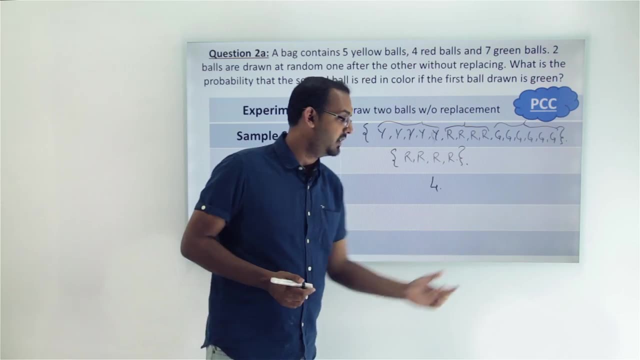 that can happen. so now the total number of events that can happen are 15, because one ball is already kept aside. so now we have a collection of 15 different balls in the bag. so the total number of elementary events that can happen are any one of these events, which are: 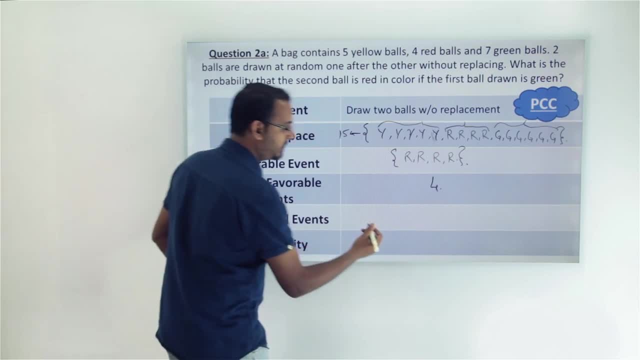 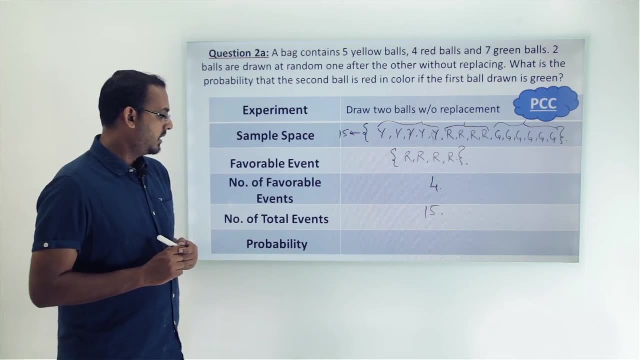 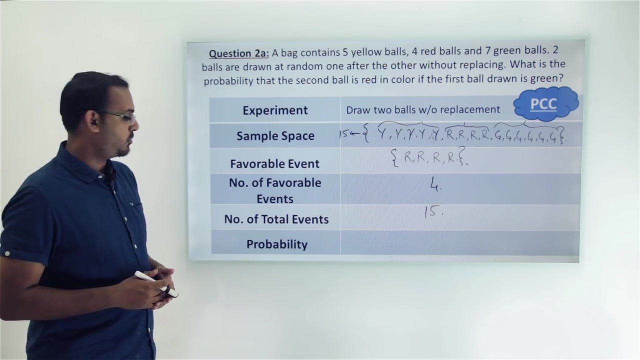 present in the sample space. so this is a total of fifteen. so the number of total events are 15. so now that now we know all the information that this question tells us. so now we have to figure out the probability. so we know that the probability is the number. 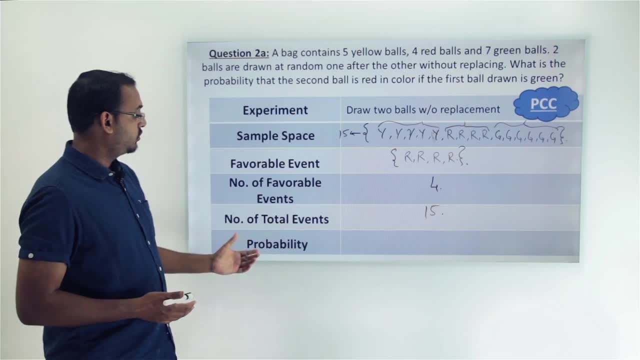 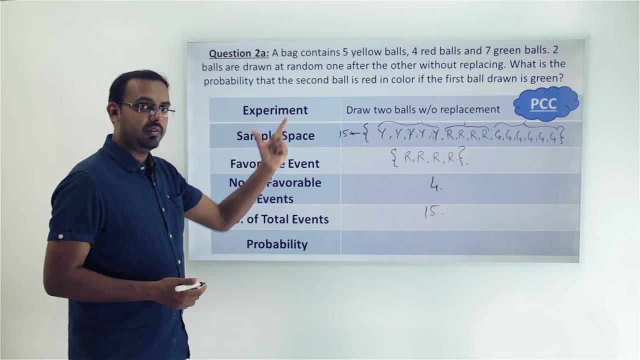 of favorable events on the number of total events. so the probability of drawing the second ball is being red in color is the number of favorable events to that event, which is four upon the number of total events that can happen. so the number of total elementary events that can happen are all the. 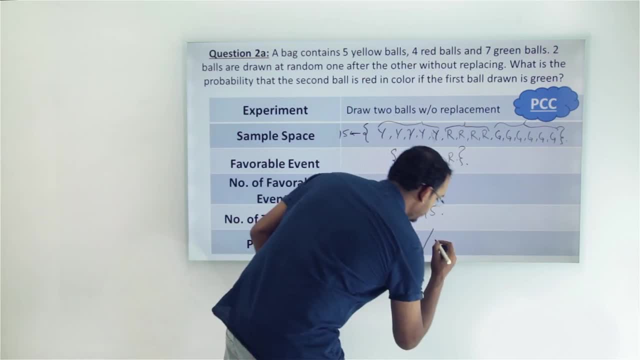 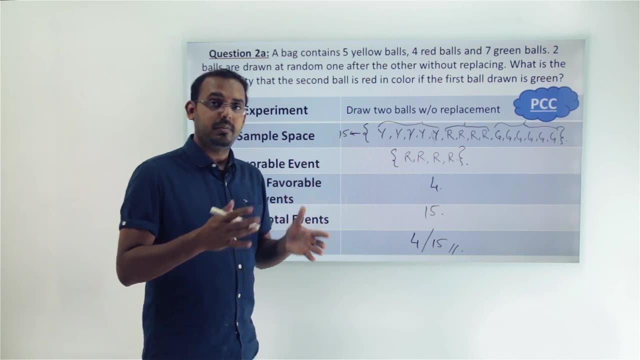 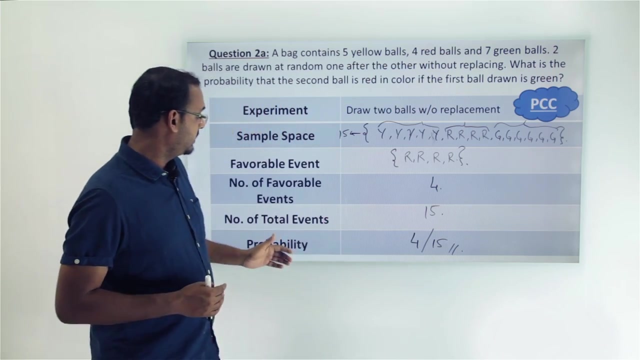 elements in the sample space, which is 15. so the probability of drawing the second ball out of the bag as a ball red in color, if the first ball drawn from the bag was green in color, turns out to be four by fifteen. so now let's try to. 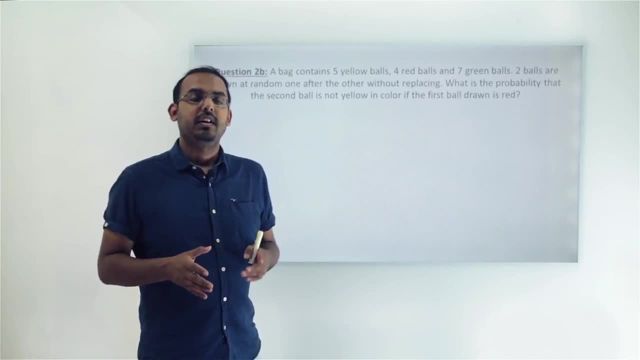 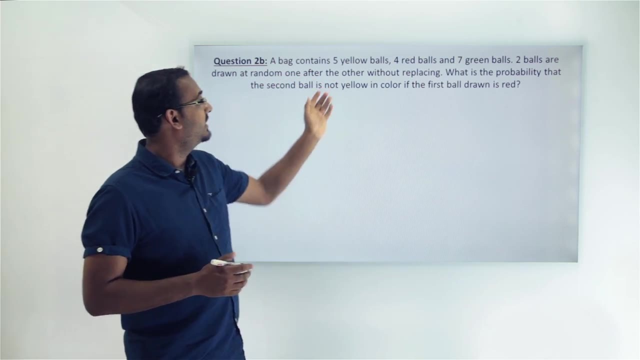 solve another type of question which can be formed in the same kind of experiment. so let's have a look at the question. so the question here says that a bag contains five yellow balls, four red balls and the seven green balls. so this is the similar. this is a very 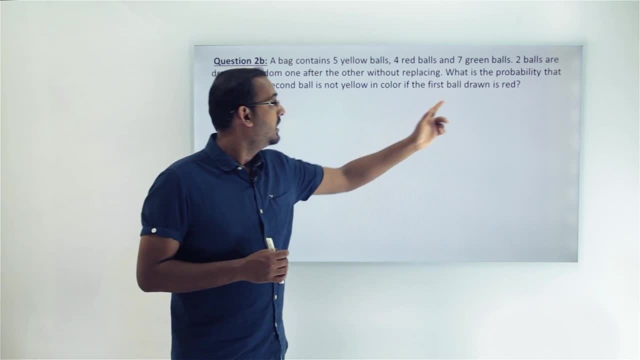 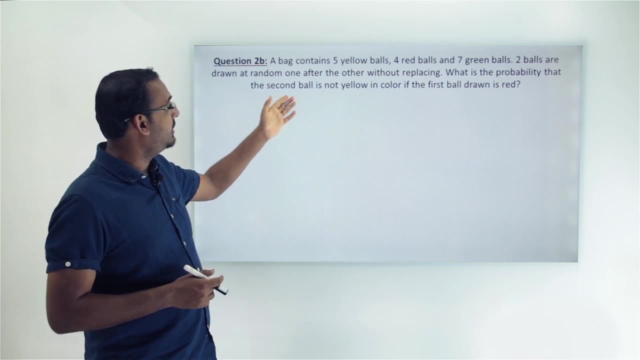 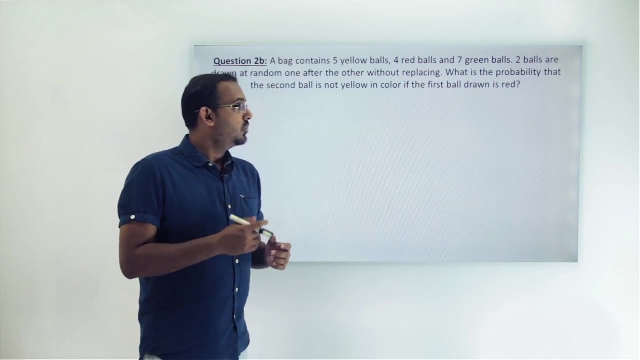 similar setting to what we had in the previous question. now, two balls are drawn at random, one after the other, without replacing. what is the probability that the second ball drawn is not yellow in color if the first ball drawn is red? so here we are. we have been asked to find the 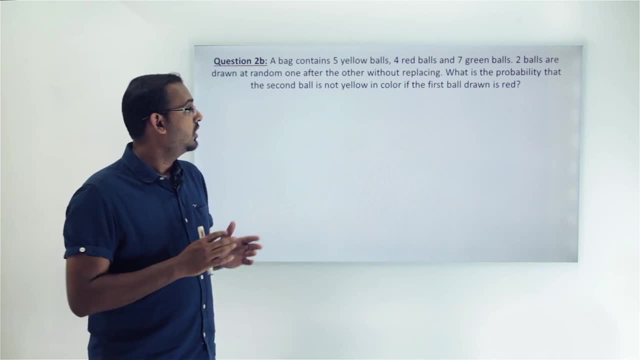 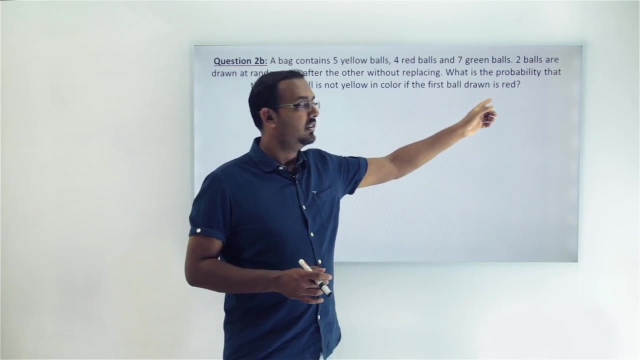 probability of the second ball that we draw to not be yellow in color. so it can be green or it can be red in color, but it should not be yellow in color after drawing the first ball, which is red in color. so now let's create the PCC here. 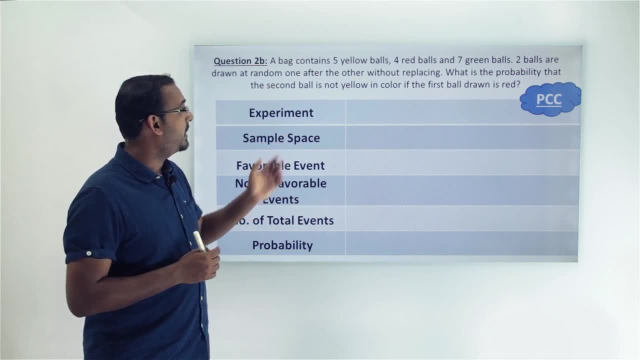 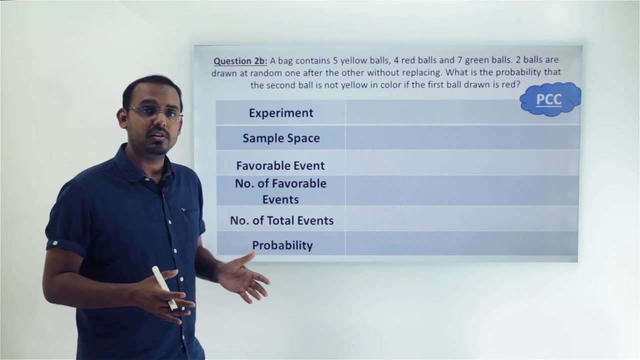 again and try to analyze this question. so the experiment that we are doing here is again the same. so we have the same setting and we have a bag in which we have put these 16 balls and we pick one ball out at random and then we keep it. 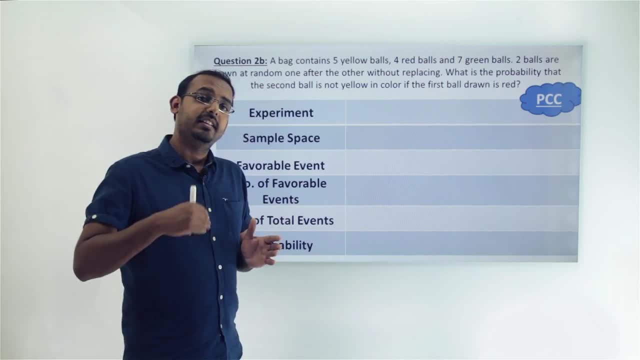 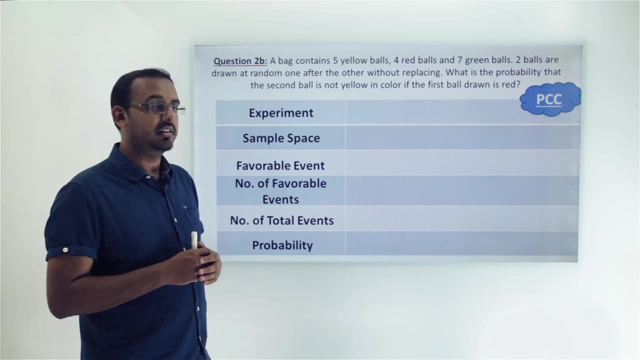 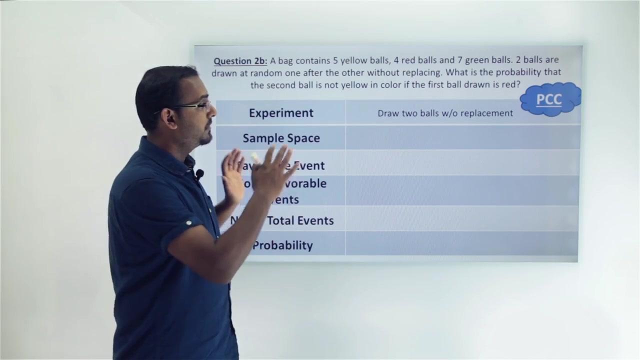 aside, and once we keep it aside, then we are trying to draw another ball from the bag. so the experiment that is here, that that will put in the PCC here, is the same. so draw two balls at random. now the sample space of this particular question is again going to be very similar to. 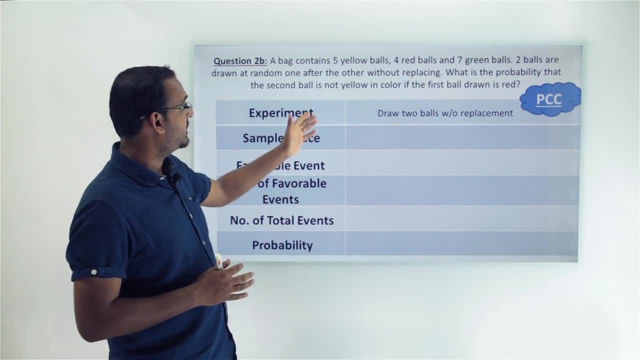 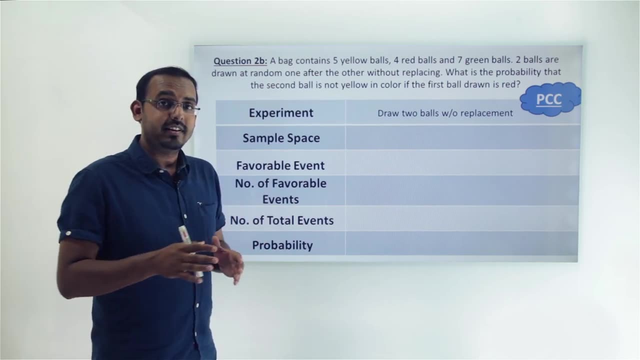 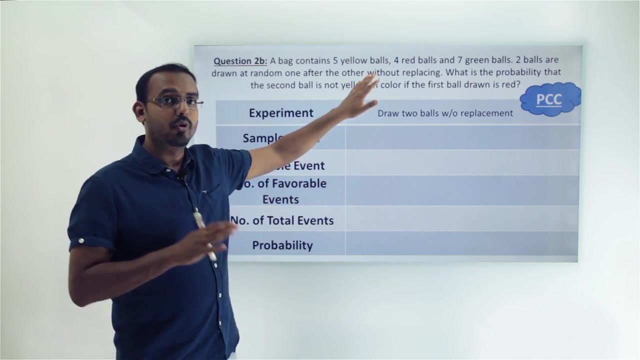 what it was before. so here the question tells us that the first ball that we have drawn is red in color. so now, after drawing the first ball, the balls that will be left with will be five yellow balls, three red balls and seven green balls, because there are four. 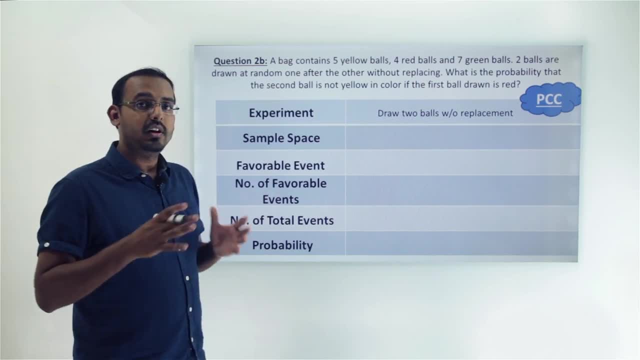 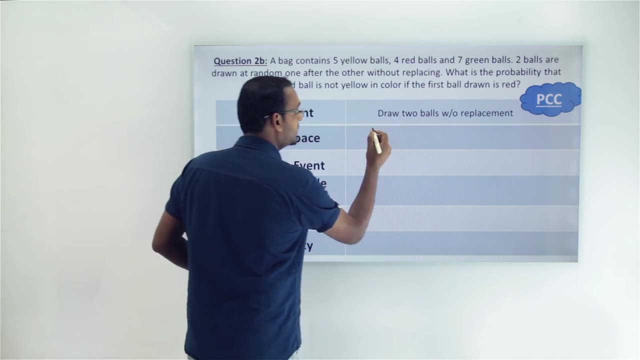 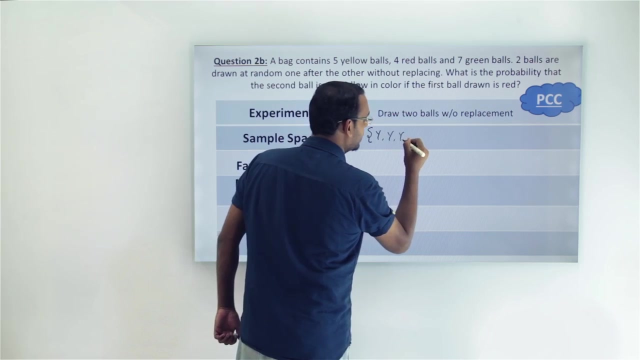 red balls and we have drawn one red ball out. so the total number of balls will be there now, after drawing one out, will be 15. so the sample space that will be here is the five yellow balls are still remaining. so the five yellow balls. then we have the seven green balls, which 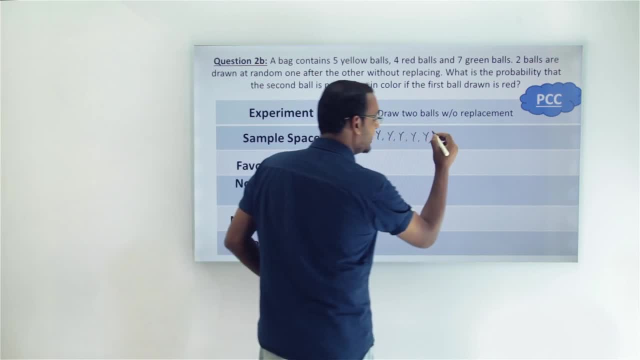 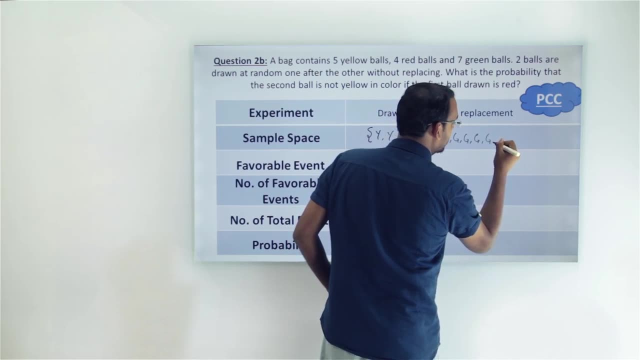 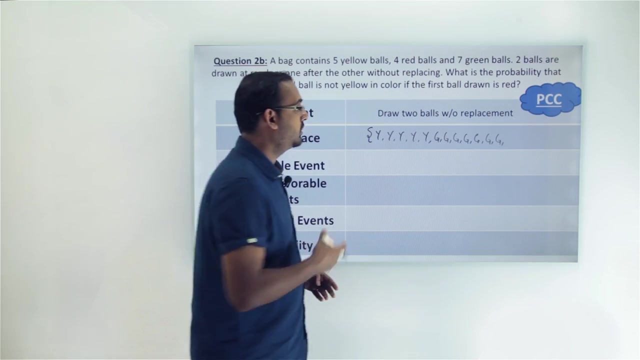 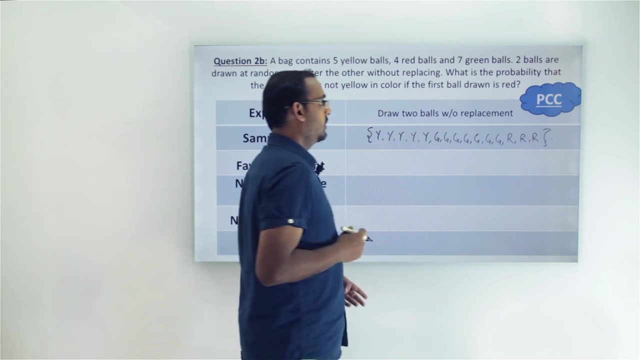 are still in the bag. we haven't drawn a green brawl out, so these seven green balls are there in the bag, and out of the four red balls that we have drawn, one already. so there are three red balls that are remaining and we have. So the next time we draw a ball out, these are the options that we'll have. 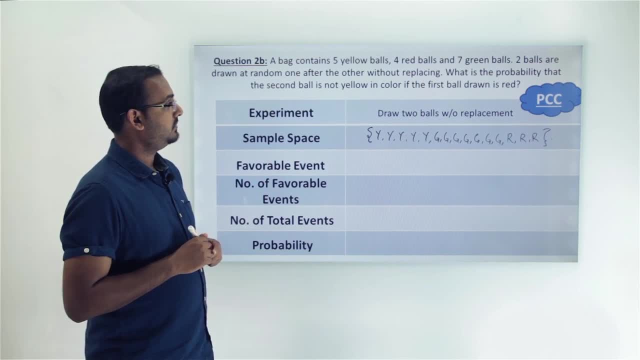 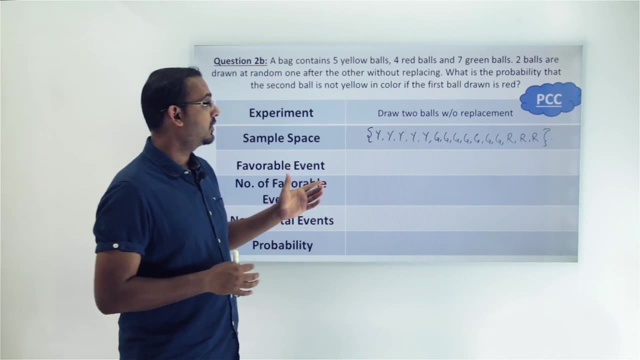 So now, what is the favorable event here? Think about it. So now what we want to do is not draw a yellow ball, So we can either draw a green ball or we can draw a red ball, But yellow ball is not favorable to us. 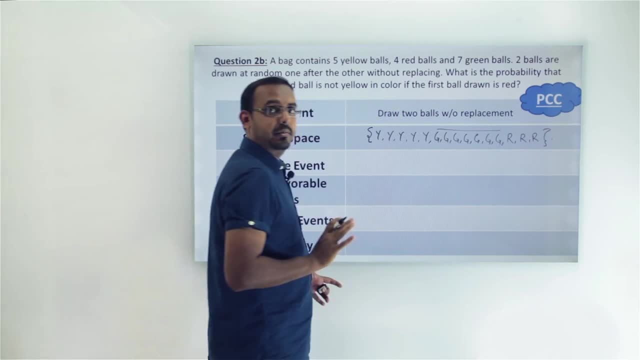 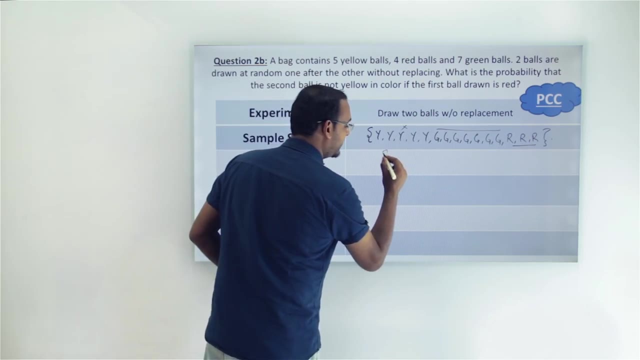 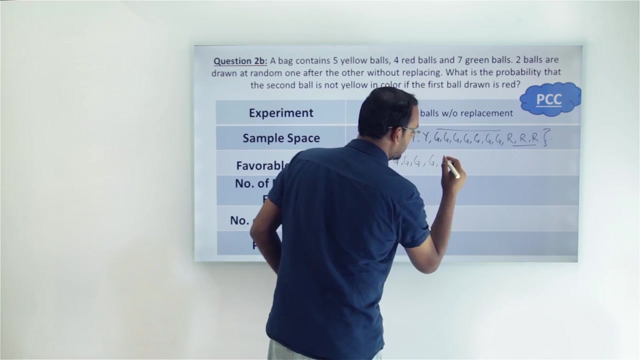 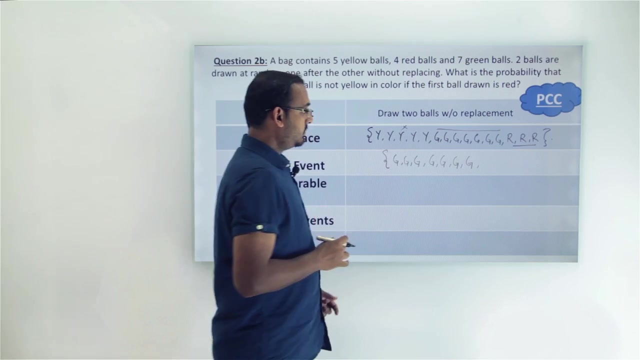 So, as we can see, there are 7 green balls left in the bag and 3 red balls left in the bag, and all the yellow balls are not favorable. So the favorable event set that we have is going to contain the 7 green balls and it can contain the 3 red balls. 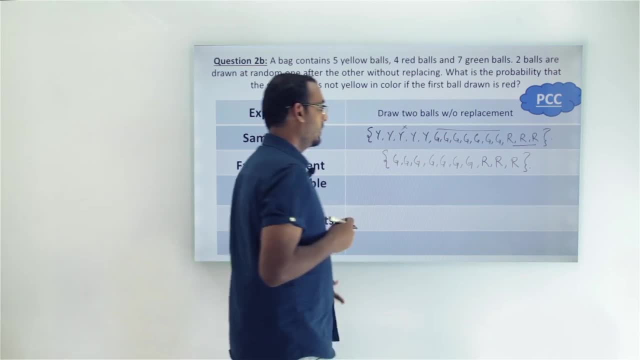 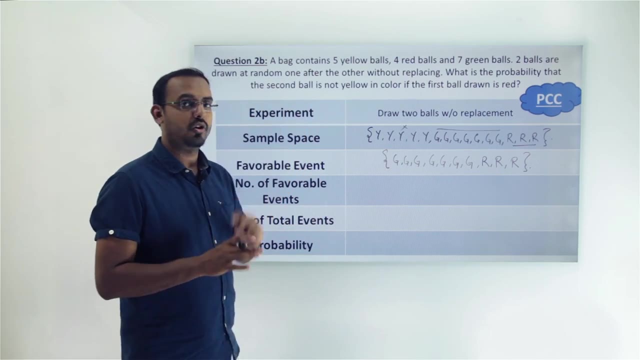 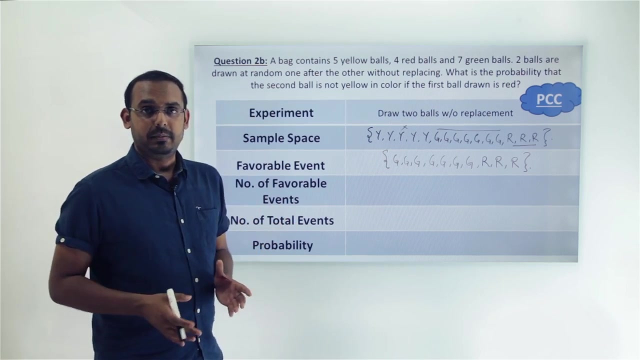 So this set represents all the cases which are favorable to our case which is not drawing a yellow ball. So now the number of favorable events are the number of elementary events which are present in the favorable event set. So we have 7 green balls plus 3 red balls. 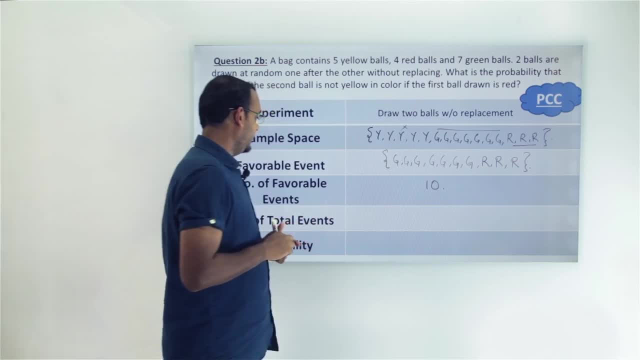 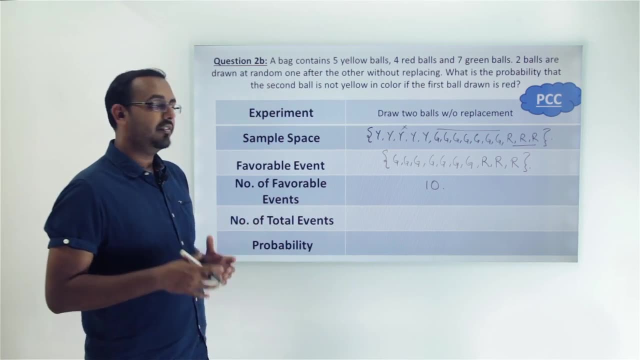 So a total of 10 balls are present in the favorable event bag. 5 green balls are present in the favorable event bag 6 green balls are present in the favorable event set. So if we draw any of these 10 balls, we can say that we have a favorable event.